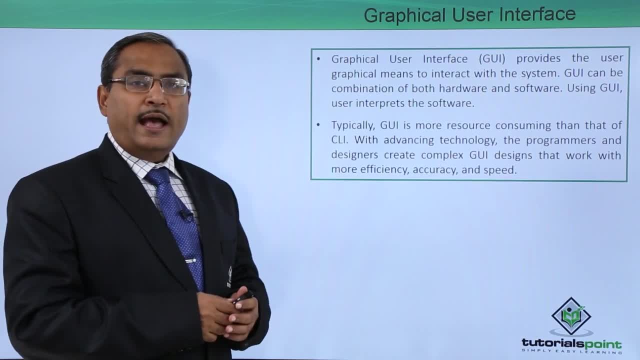 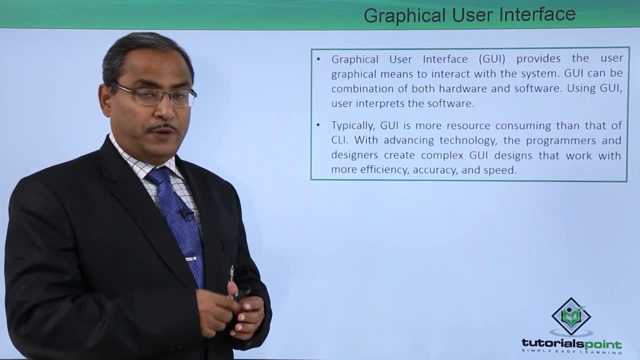 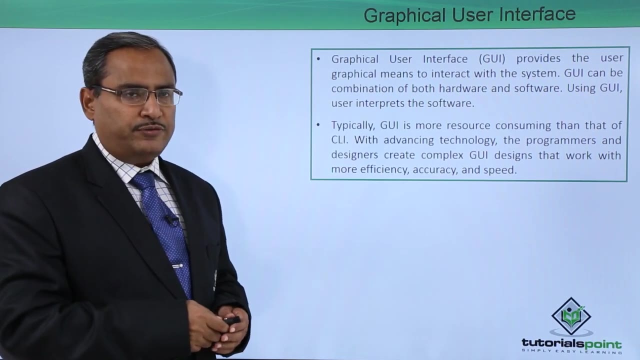 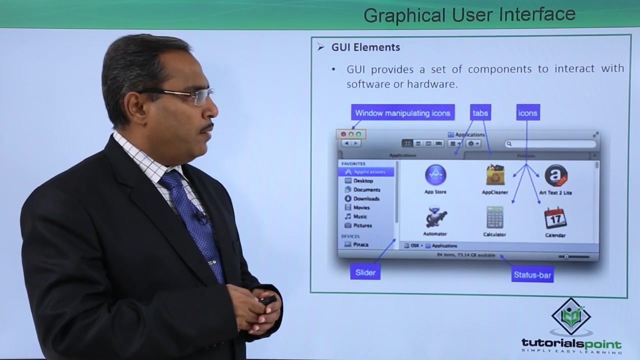 designs that work with more efficiency And with more speed. so obviously this GUI designing is a challenge because the user should feel a very comfortable and convenient and user friendly environment to interact with the software. So at first we are going for the GUI elements. So GUI provides a set of components to interact with the 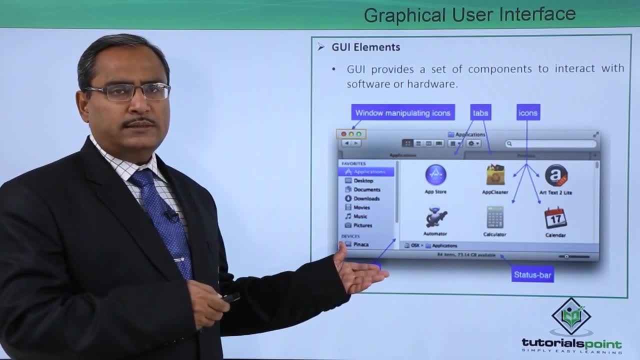 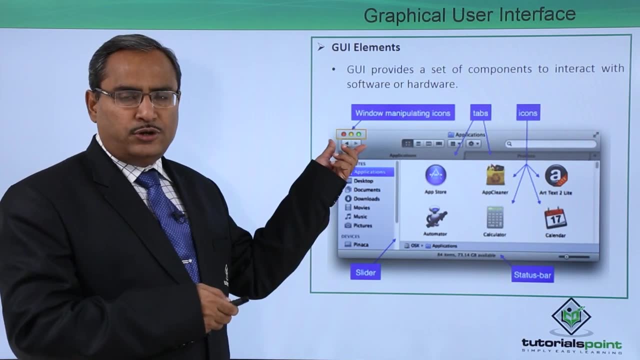 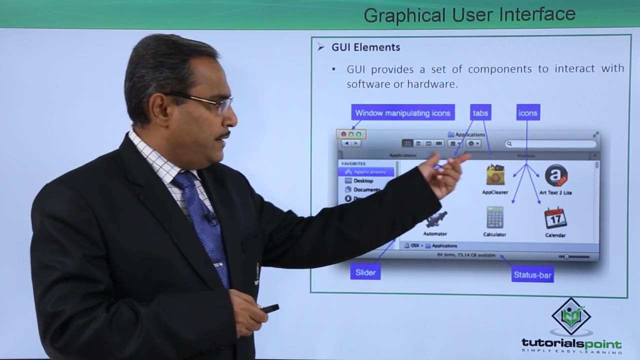 software or the hardware. So here we have shown you one sample window. So here you can find that we are having this window manipulating icons. We can maximize the window, we can resize the window, we can close the window. So these are the window manipulating icons are there. 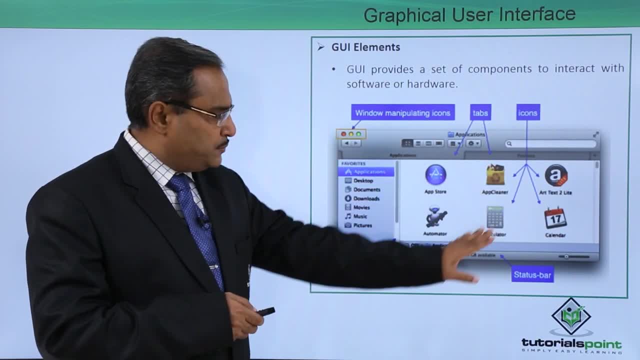 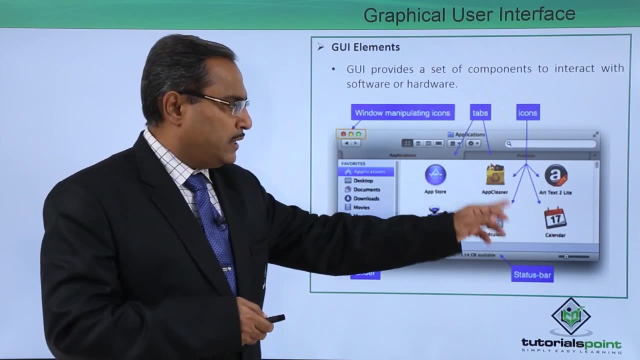 Here we are having multiple tabs. So if you click on a certain tab, the respective icons will be coming. If you click on another tab, the another set of icons will be coming. So here we are having the respective icons. So icons are nothing but small pictures. are there? 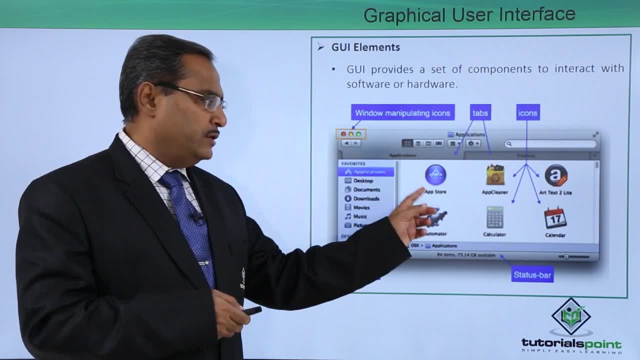 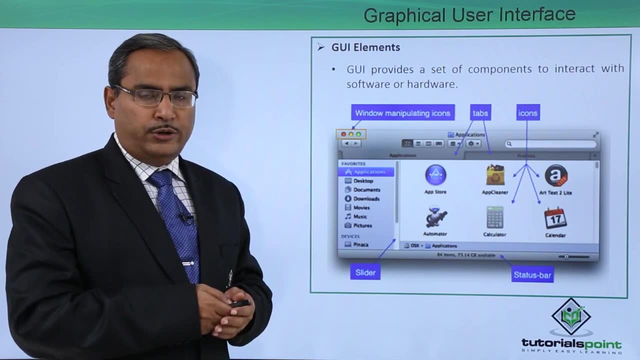 So on this particular pic, we can click using our mouse. mouse is a hardware and these are the respective icons are there, You can double click on them and obviously we know that when the daspected operation will be performed. Other is also, you can have that touch screen. 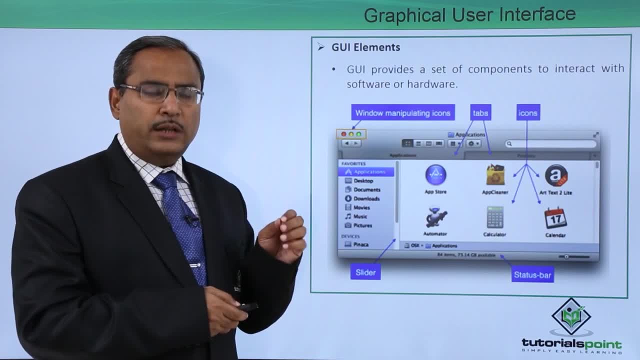 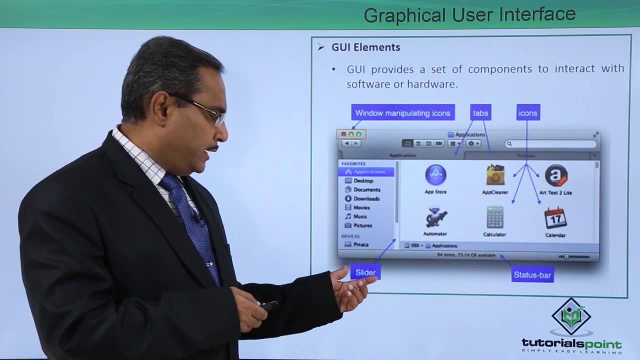 where you can touch the screen and the respective icon will respond. So here we are having multiple defendant options are coming in the side pane. So here we are having the slider and here we are having this stand right. here we are having the center white screen and this is the mouse which is showing below the screen. 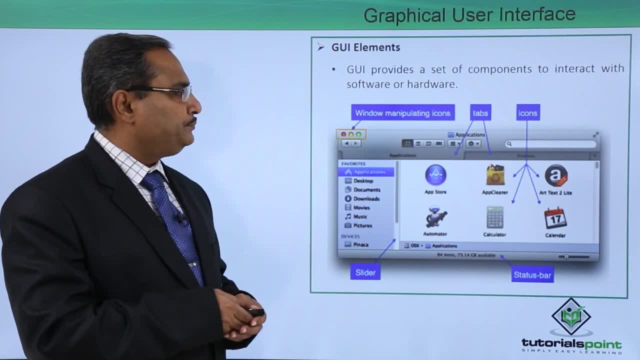 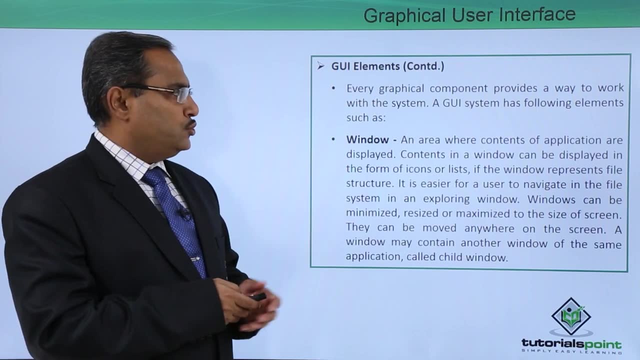 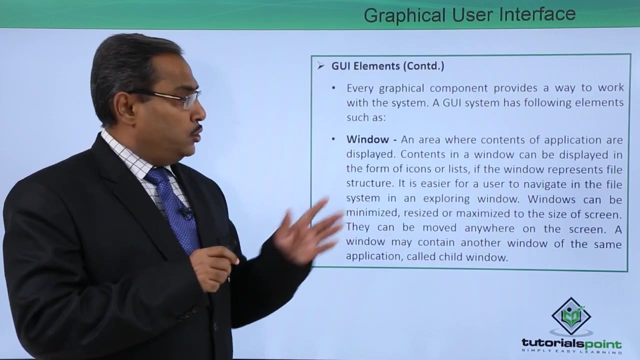 which will be showing the status of the software. So every graphical component provides a way to work with the system. So here we are having the following elements we are going to discuss on. So first one, we are considering the window, So a area where contents of the application, 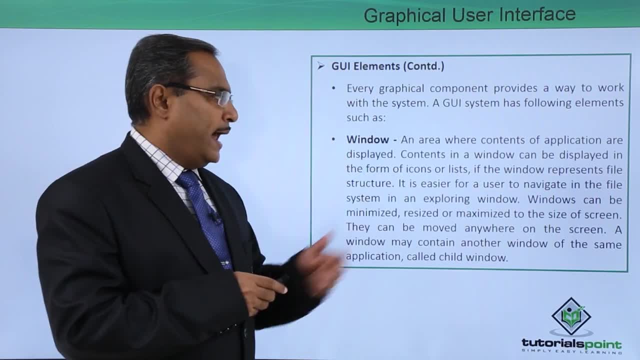 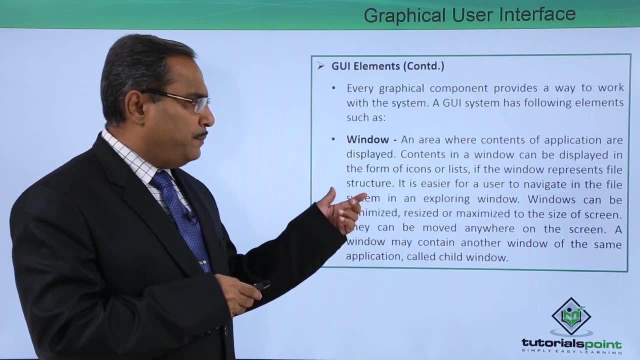 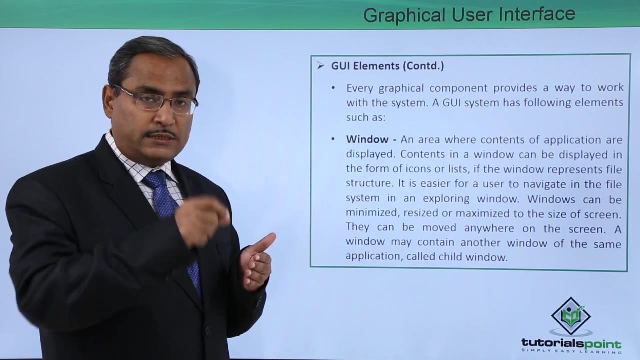 are getting displayed will be known as the window, and contents in a window can be displayed in the form of icons or in the form of lists. If the window represents the file structure, then we can having the multiple files and what are the respective folders and sub folders. 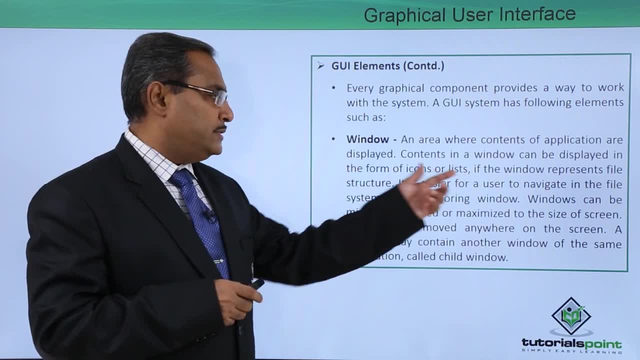 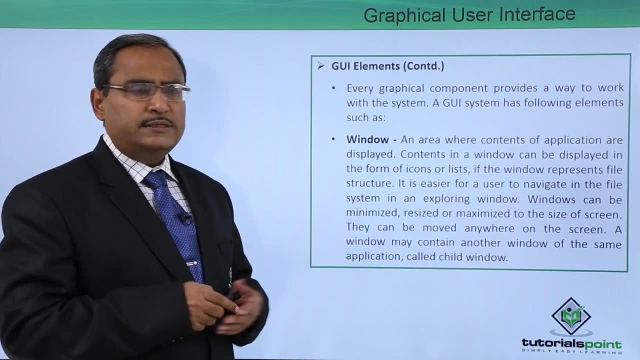 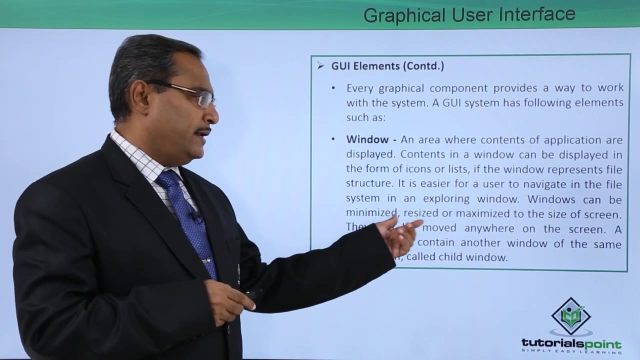 they will be coming accordingly. So if the window is representing a file structure, then the content of the window can be displayed in the form of a list or the set of icons. So it is easier for a user to navigate in the file system in an application. So the 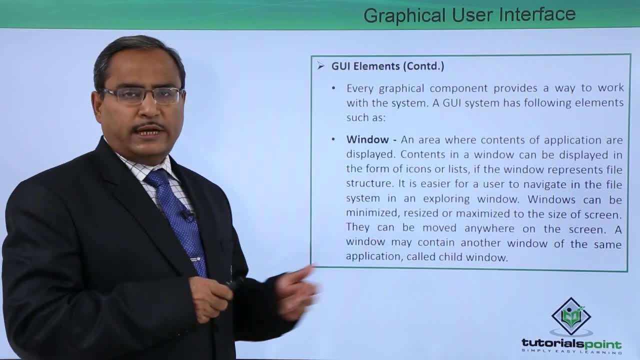 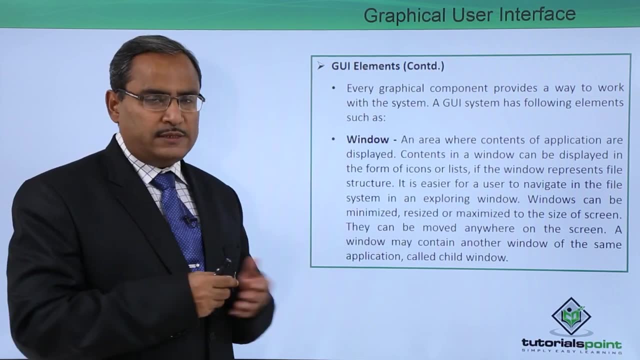 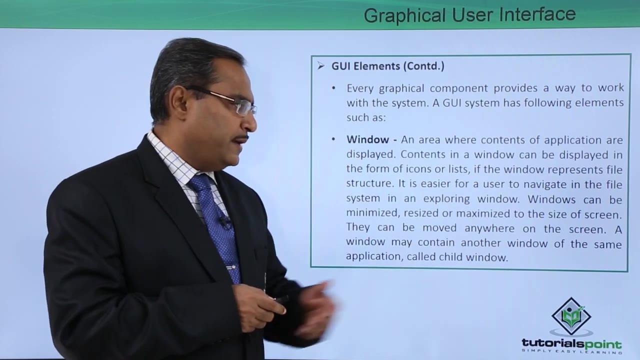 exploring window. so here we are having window that is a Windows Explorer, if you consider the windows operating system. we are having the Windows Explorer where you can explore a file system through that option to that window. So windows can be minimized, resized and maximized with the size of the screen. They can be moved anywhere on the screen. 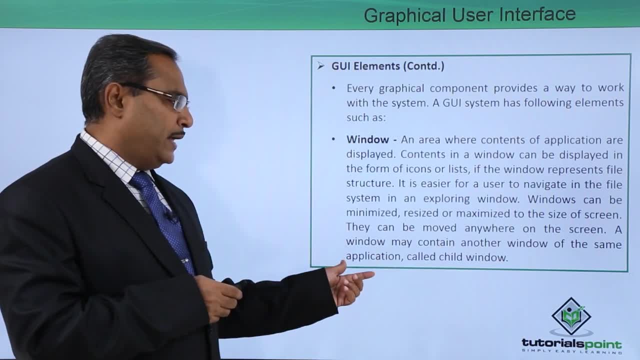 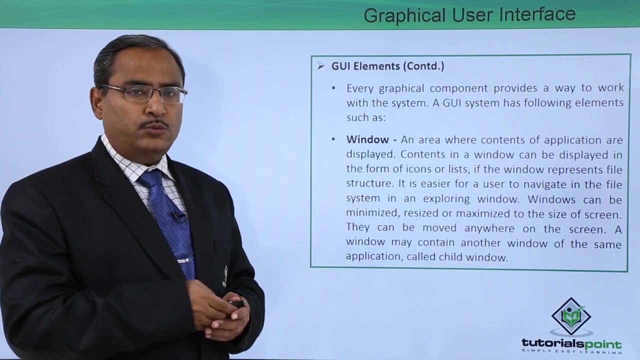 a window may contain another window of the same application called a child window. So these are the different aspects of the child window. Thank you of the g a component. that is our window. next one we are going to discuss tab. so if an application 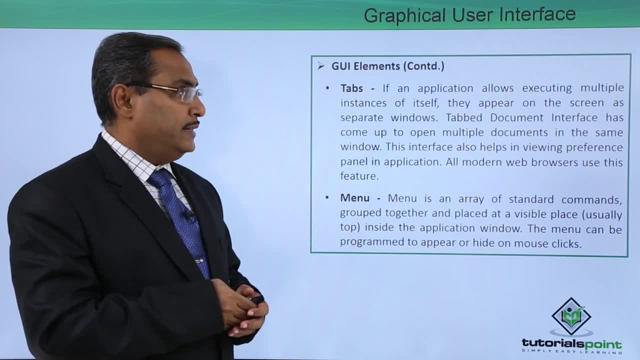 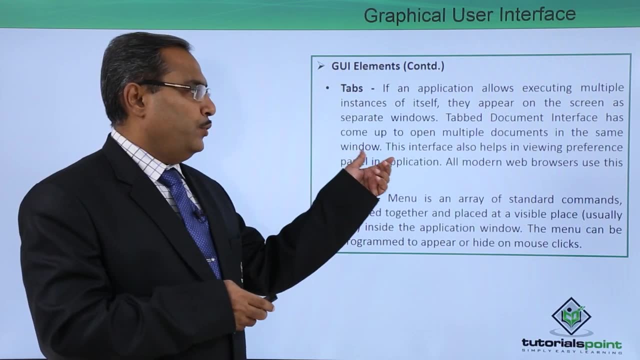 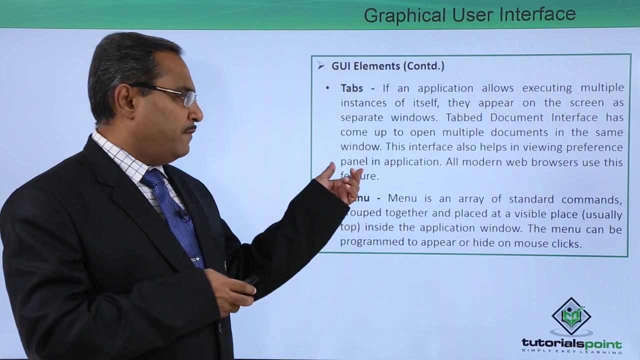 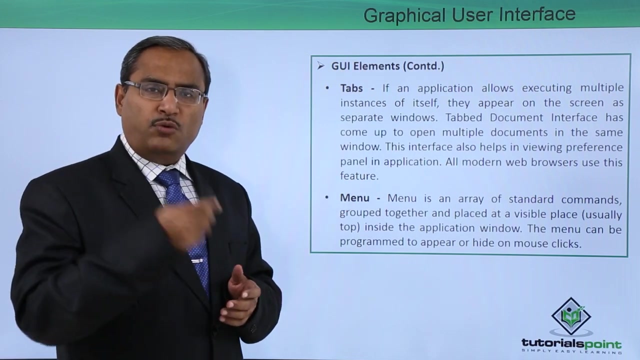 allows executing multiple instances of itself. they appear on the screen and separate windows tab document interface has come up with to open multiple document documents in the same window and this interface also helps in viewing the preference panel in the application. and all modern web browsers use these features. we know that if you open one web browser then 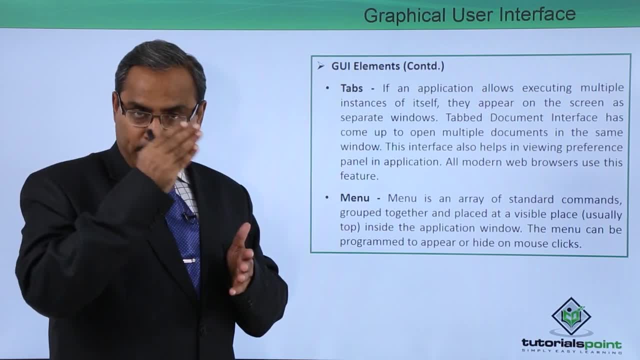 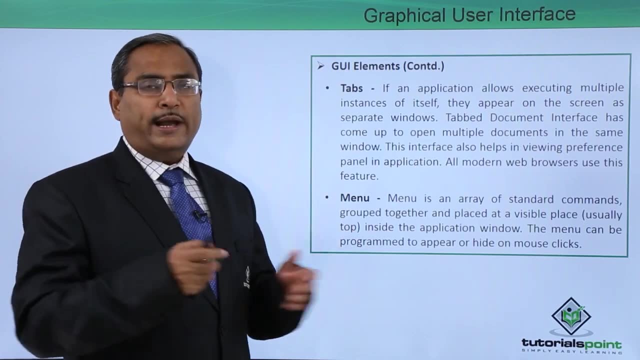 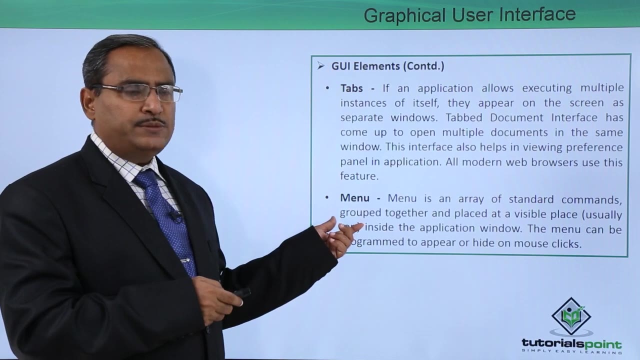 we can. we can see multiple different websites and they will be coming in different, separate tabs. so we can close a tab, we can create a new tab where, within the same window, we can have multiple different websites and their respective displays. next one: we are considering the g? y component, that is, menu. so menu is an array of standard commands grouped together. 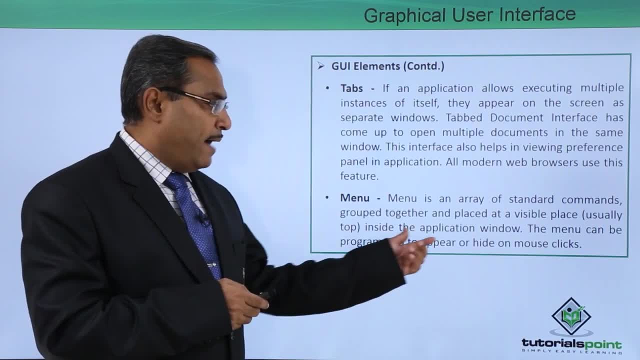 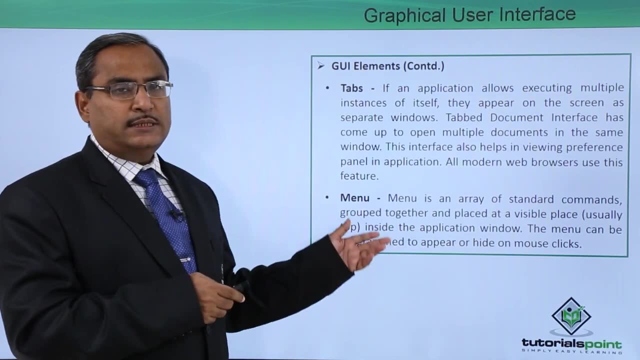 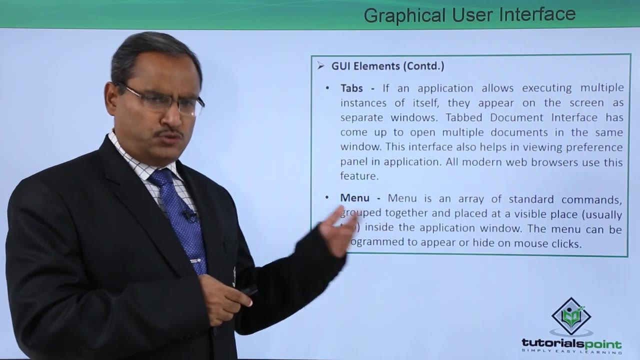 and placed at a a visible place Inside the application window. the menu can be programmed to appear or hide on mouse clicks. So this is the menu. So we can have different kinds of menus are there? We are having the menus and submenus, the context menu. So so many different types. 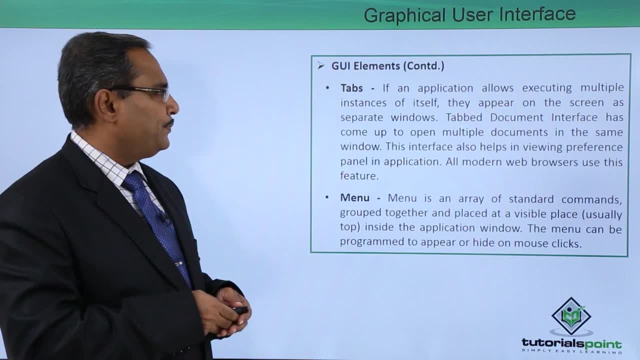 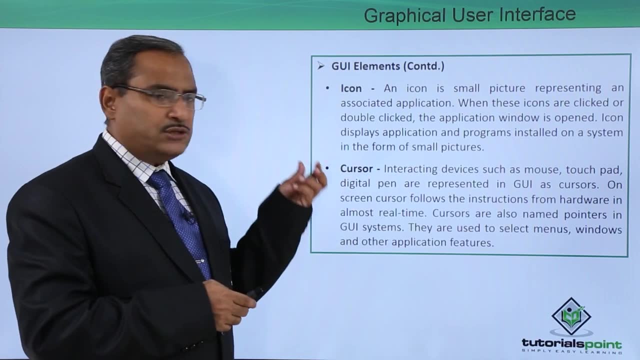 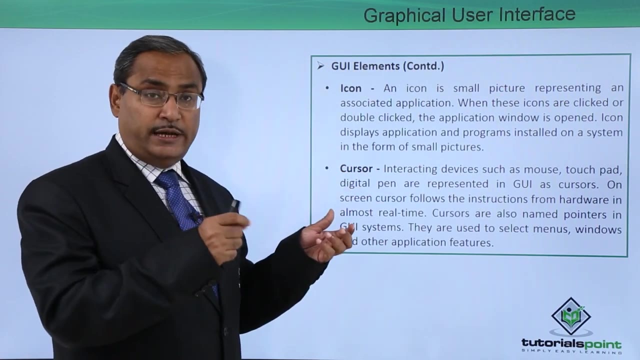 of menus are there where multiple options can get listed. So next one we are considering is icon. An icon is small picture representing and associated with an application, And when these icons are clicked or double clicked or using the touch screen- if you touch that- 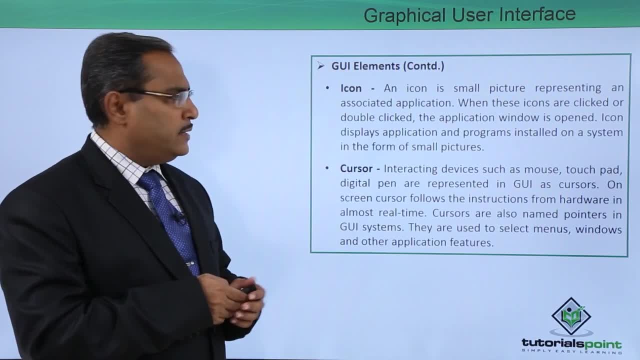 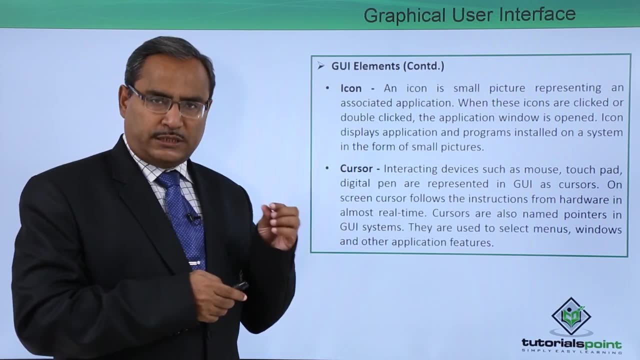 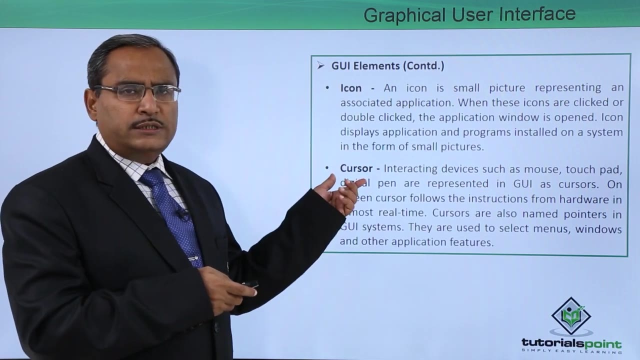 respective icon, the application window will be opened. The icon displays application and programs installed on a system in the form of small pictures. So icon will be having a small picture and along with that there may be a text line. Next one we are going to discuss. 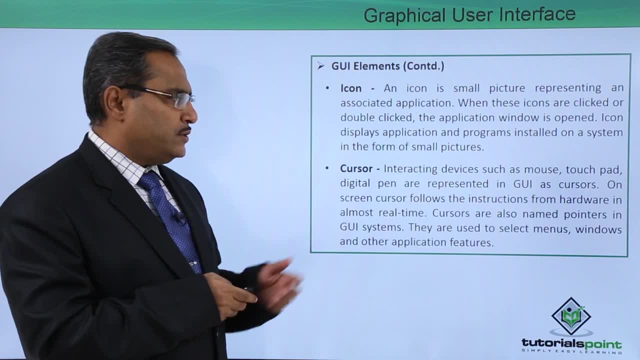 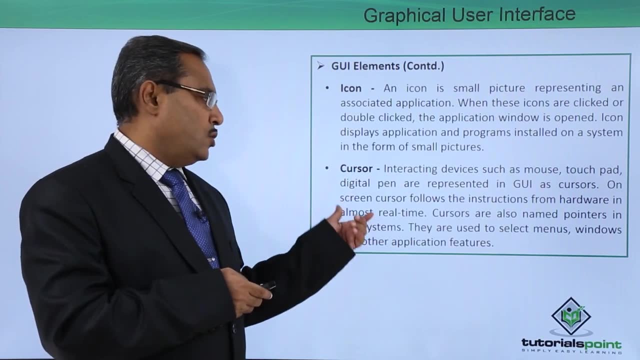 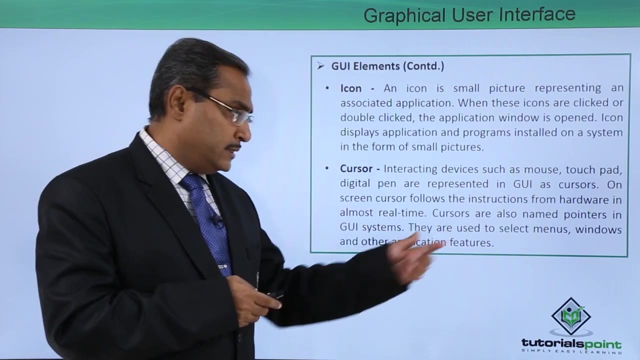 that is our cursor. So interacting devices such as your mouse, touchpad, digital pen are represented in GUI in the form of a cursor On screen. cursor follows the instruction from hardware in almost real time And cursors are almost are also named pointers in GUI systems. 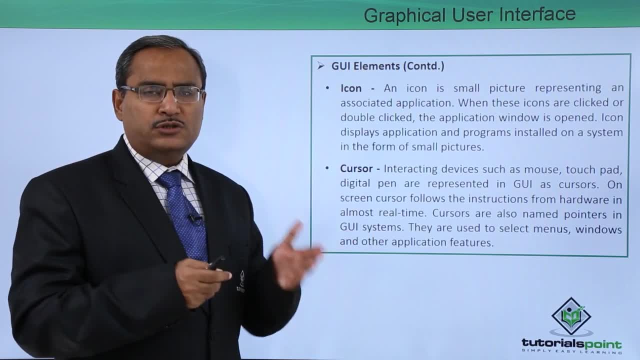 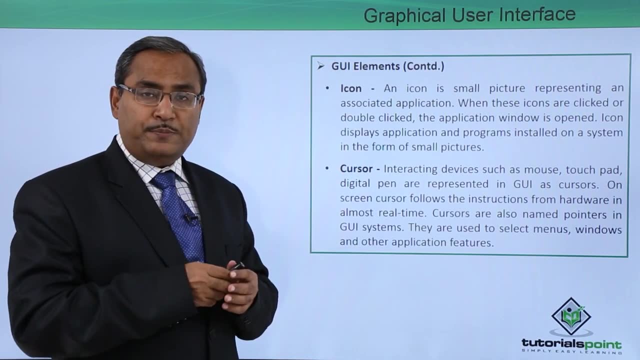 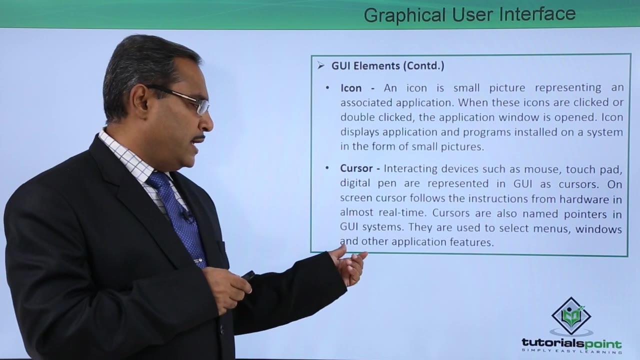 So whenever we are finding, say, just consider one text box where one cursor is blinking and if we type a text Immediately, we get the response from the system and the corresponding text will appear whatever we have typed on that respective text box. So they are used to select menus- windows. 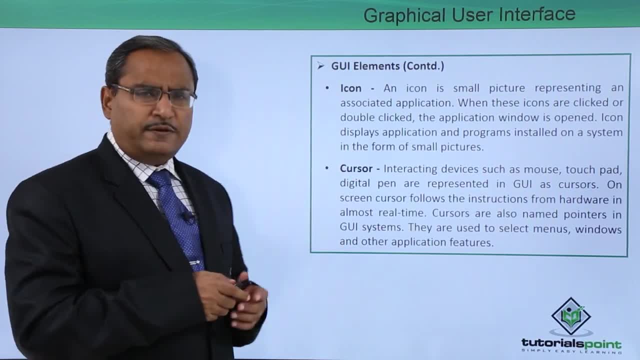 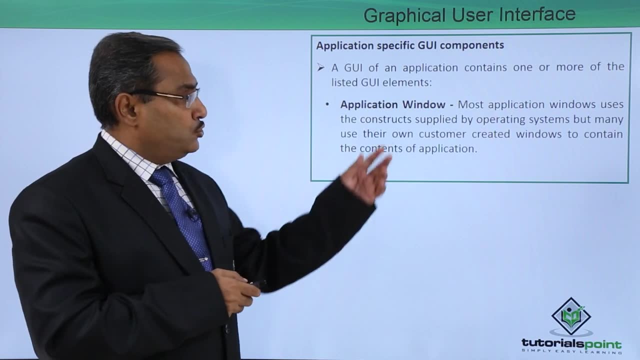 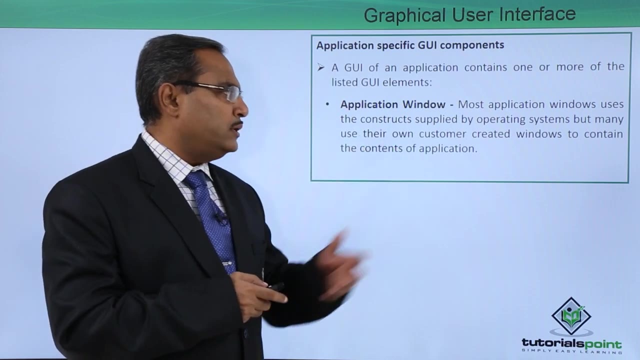 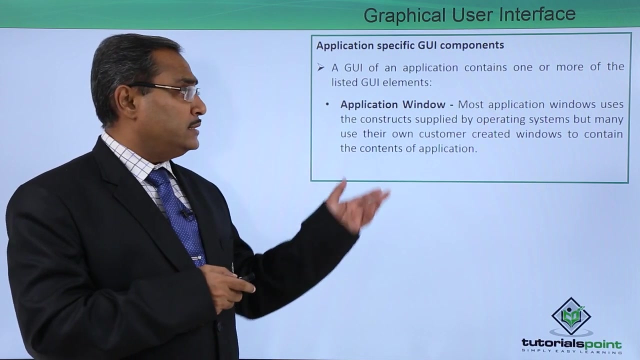 and other application features. So these are the different GUI components we are discussing here. So now let us consider one application window. So most application windows uses the construct supplied by the operating system, but many use their own customer created window to to contain the certain components of the application. So this is known as the respective 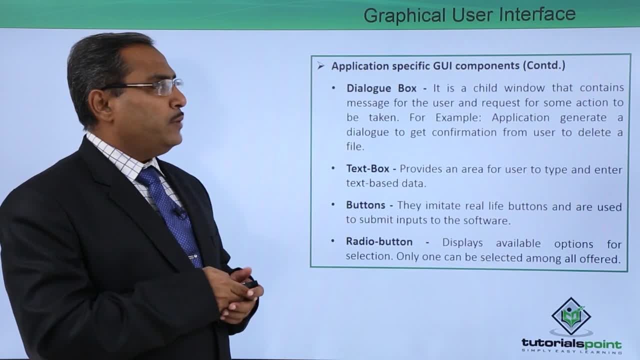 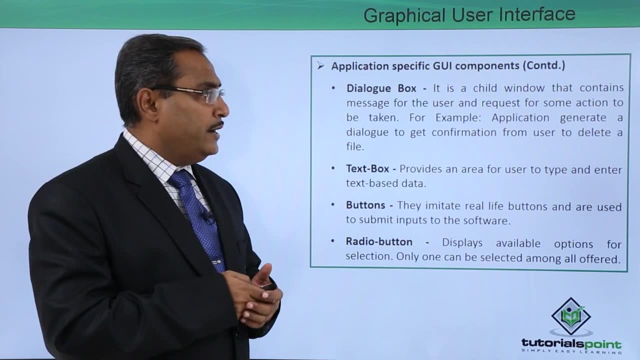 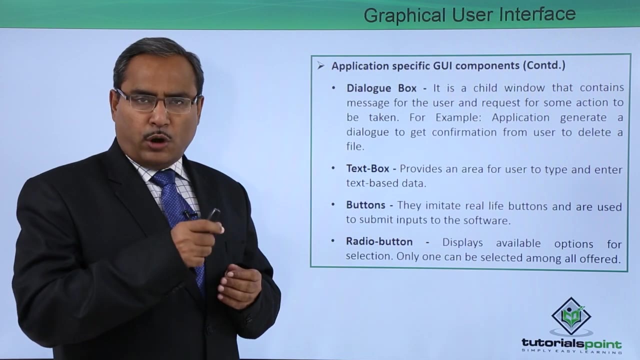 application window. Next one we are going to discuss, that is our dialogue box. So it is a child window that contains message for the user and request for some action to be taken. So let us suppose that is one dialogue box which is containing options, say abort, retry, cancel or say ok. 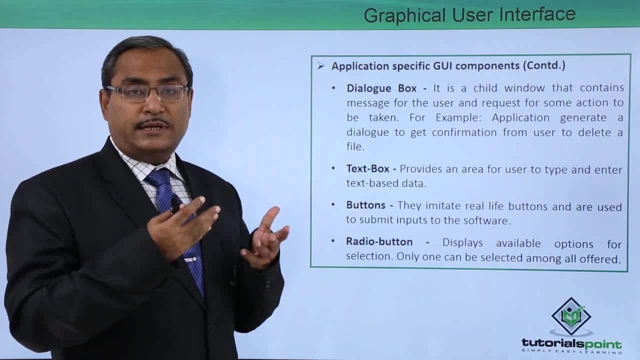 So these are the dialogue box which usually appear on the screen. So let us suppose that is one dialogue box which is containing options, say abort, retry, cancel or say ok. So these are the 4 available options which usually appear on our screen. Now, as a user, we should 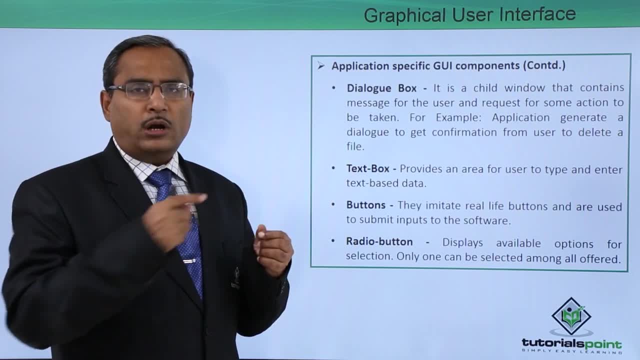 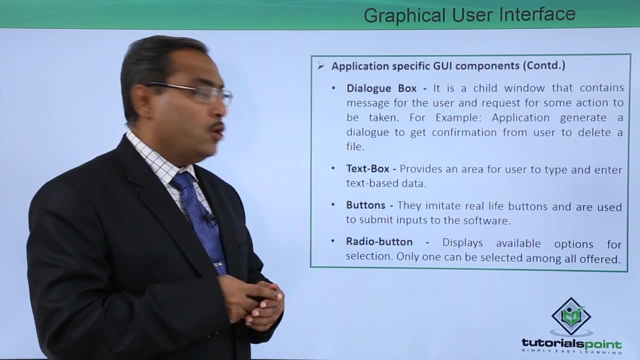 interact whatever the options are given. we can interact with one of the options according to my choice. For example, application generates a dialogue to get confirmation from the user whether it should delete a file or not. Next one, we can consider the text box that provides an. 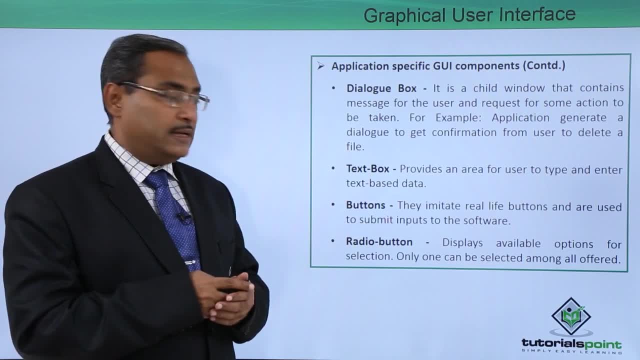 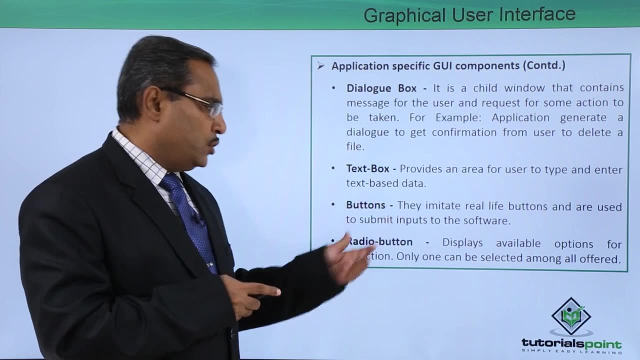 area for user to type in the text based data. Next one is the buttons so that imitate real life buttons and experiments. So these are area where the- misschien an important component- are used to submit inputs to the respective software. You can click on the button and. 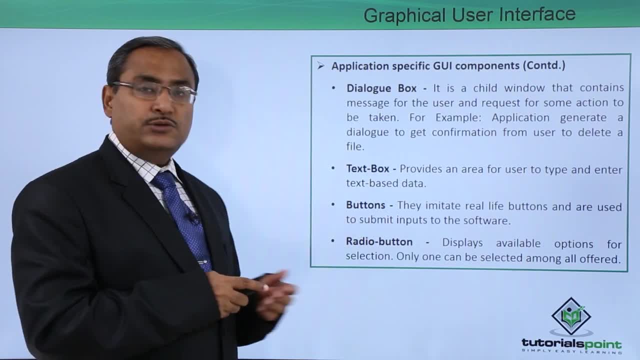 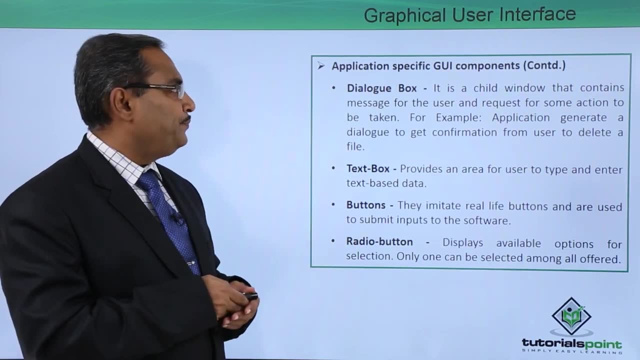 the respective operations will get list of radio buttons. So in case of radio buttons we might be having, say, two radio buttons, but either one of them can be selected at a time. We are having the check box, So function similar to list box when an option is selected. 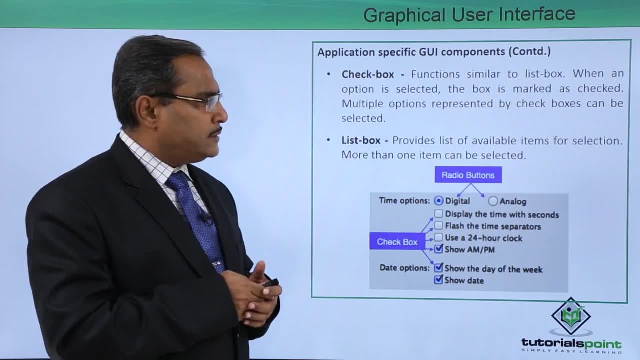 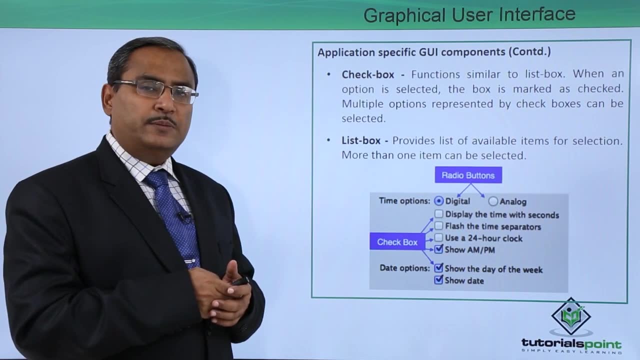 the box is marked as checked, Multiple options represented by check boxes can be selected. So, unlike your radio button in case of check box, you can select multiple check box at the same time. We are having the list box, So provides a list of available items for. 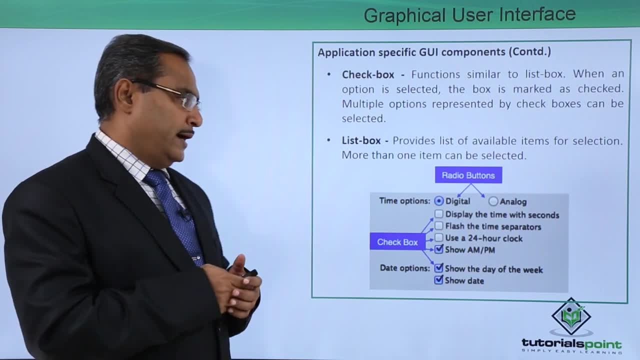 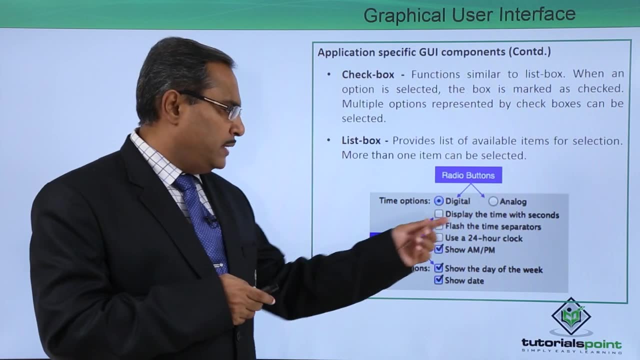 selection. more than one item can be selected at a time. So here you are getting this radio buttons. We are having two options: digital or analog. You can select any one of them. We are having multiple check box and you can select multiple number of check boxes at the 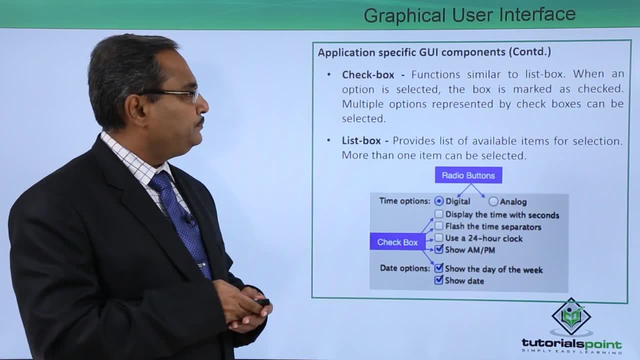 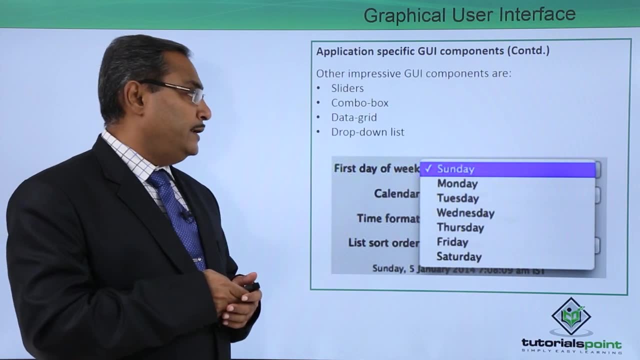 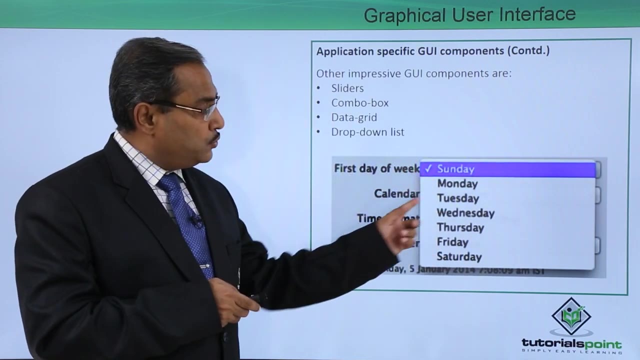 same time. So it is for the, for your reference. So other impressive GUI components are sliders, combo box, data grid, drop down list, etcetera. So here you can see that here we are having multiple days are there, you can put a tick. 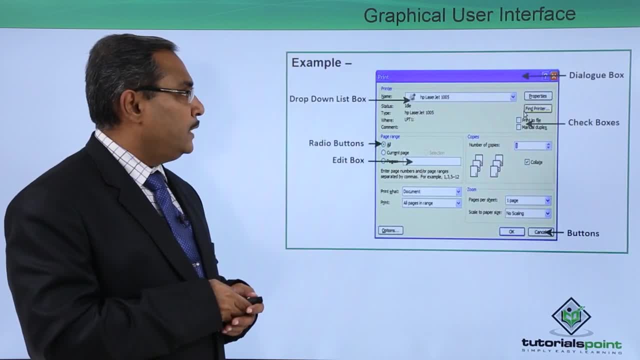 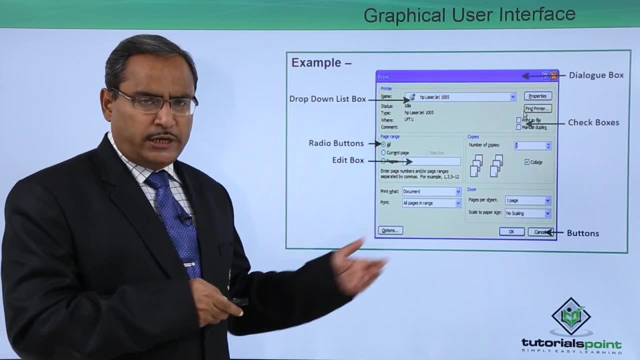 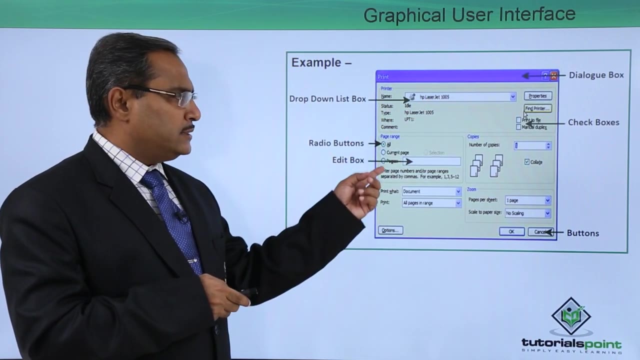 according to your selection accordingly. So here one various, very common window which we usually get when we are trying to take some print, specially in the windows environment. So here we are having multiple things are there, So drop down list can be obtained from here. radio buttons are there, whether you want to. 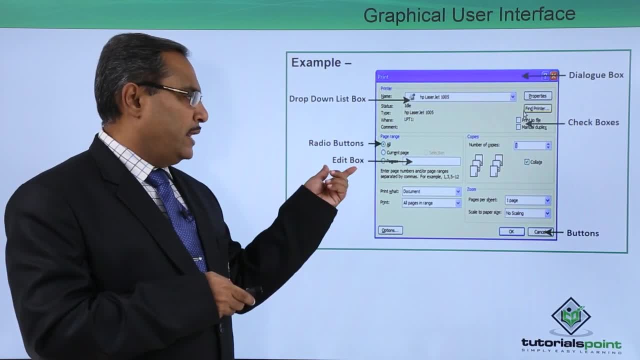 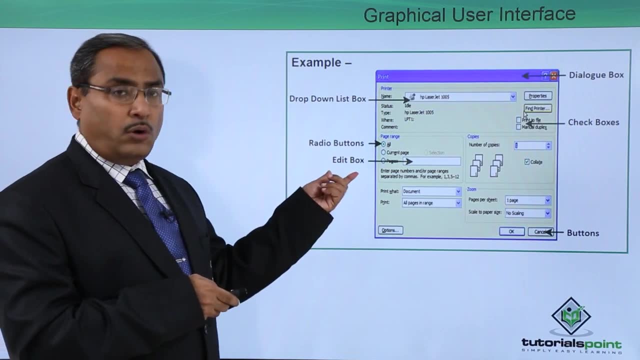 print all the pages or certain number of pages, whatever. we are having this edit box So you can type something here. So there is a from this page to that page. you can mention that one also, you can call it as a text box here. This is the check boxes you can go for. 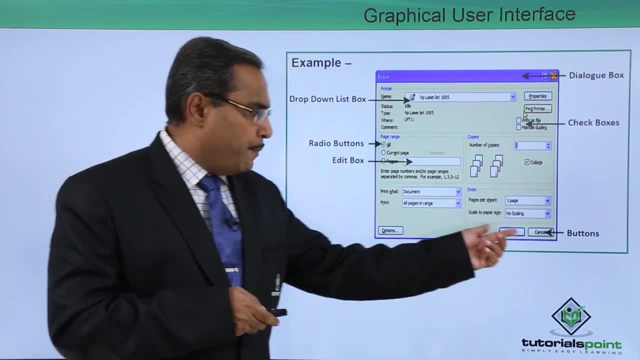 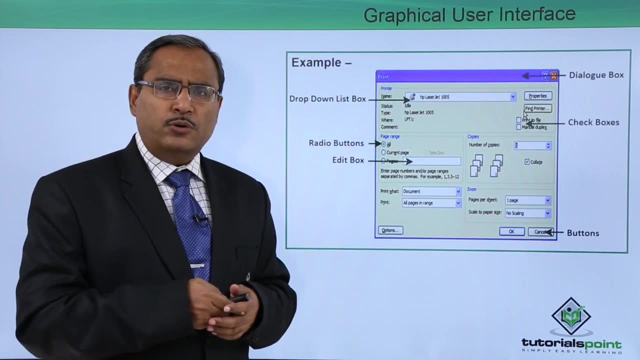 multiple selection at a time and there is a dialogue box. is there? buttons have also been shown. It is a ok or cancel, whatever you require to do. So this is a respective one sample window And where we are having multiple GUI components are deciding on this respective window. So 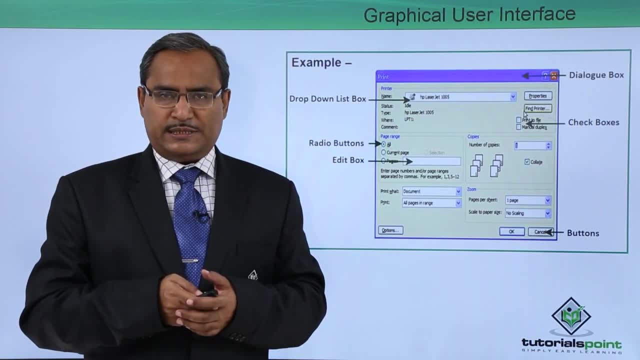 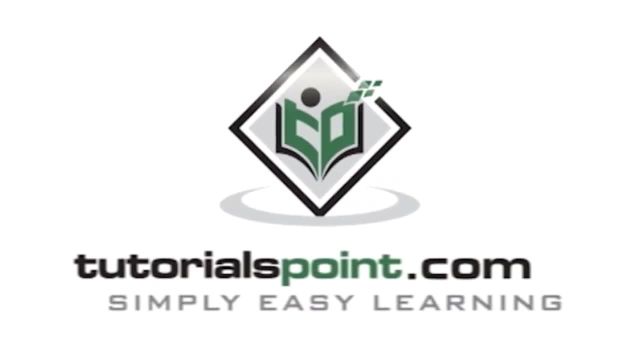 in this video we have discussed graphical user interface with some examples and diagrams. Thanks for watching this video.